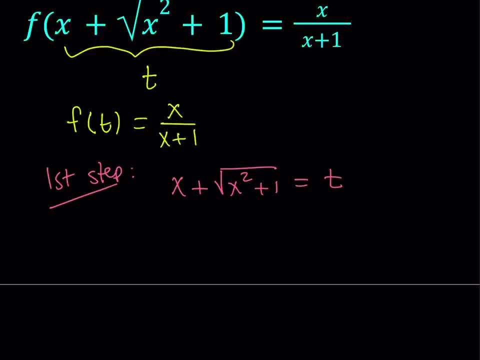 plus 1, equal to t. and then, of course, my goal is to solve for x here, so that I can write x in terms of t on the right hand side. So what am I going to do? I'll first isolate the radical. So in order. 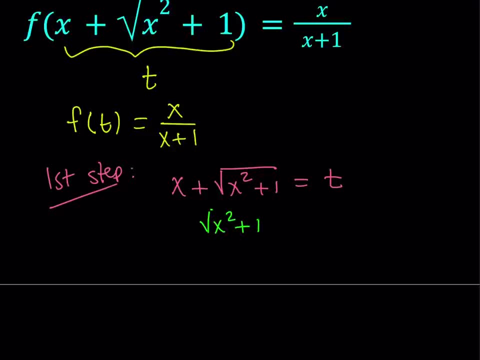 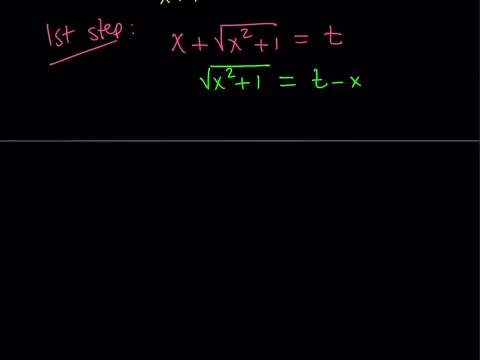 to do that. I'd like to subtract x from both sides. Let's go ahead and do that, and this is probably what looks more like Euler substitution for integrals- and obviously this is a really good method because you're going to see that it simplifies. So we're going to square both sides. 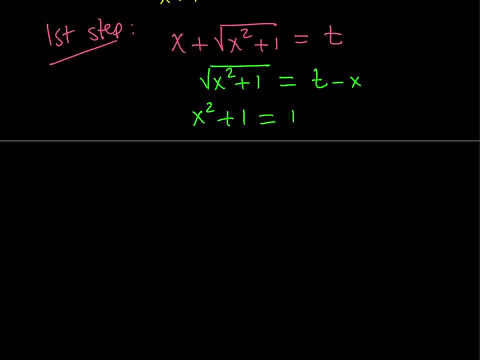 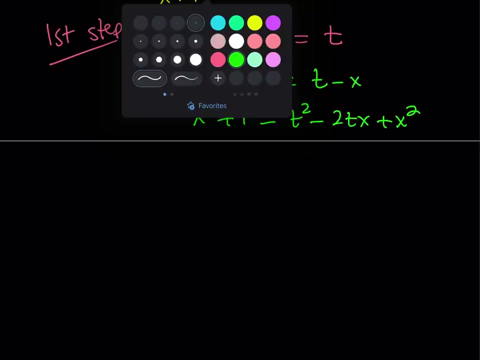 here: x squared plus 1 equals t squared minus 2, tx plus x squared. Now, the good thing about this substitution is that x squared cancels out, so we get rid of the quadratic. Let's go ahead and cancel out the t- I mean the x squared- so that we end up with this expression. Now, in this expression, 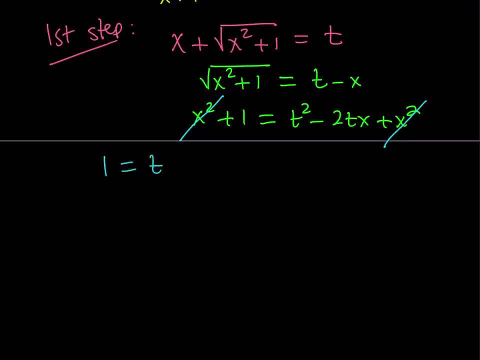 so I have something like this: 1 equals t squared minus 2 tx. Am I trying to solve for t? No, because t is already solved for here. So what I'm trying to do here is solve for x. so it would make sense if we had the x terms on one side. So let's go ahead and add 2 tx to both sides and subtract 1. 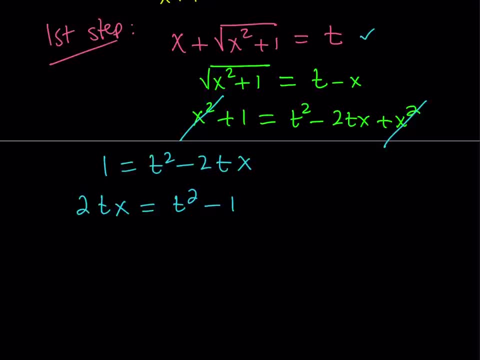 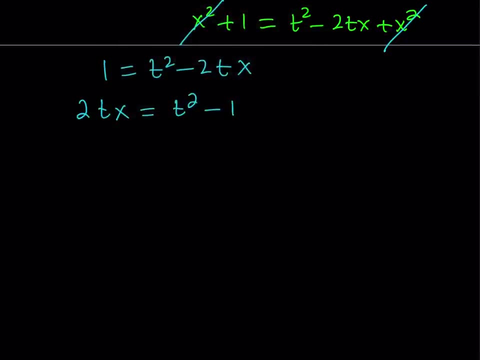 that should give me something like this: 2 tx is equal to t squared minus 1, and since my goal is to solve for x here, it will make sense to divide both sides by 2 t. I can't make the 2. u joke, right. 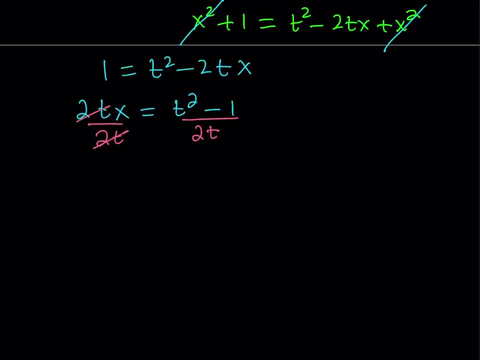 if I divide both sides by 2 t, they're going to cancel out and we're going to get x in terms of t. So this is basically the first step. So we were trying to get x in terms of t and we did. Okay, that's my first step. Now my second step involves substitution, Of course. the first step 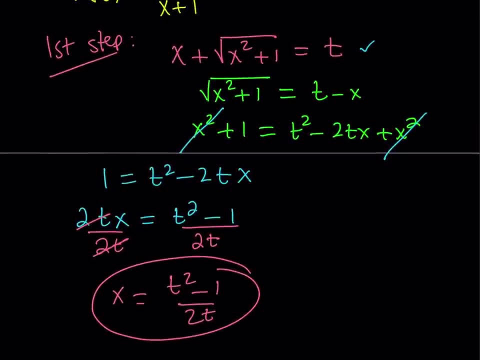 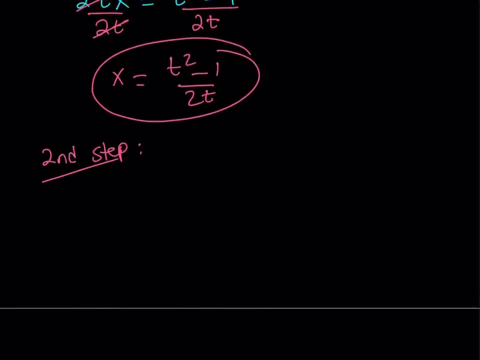 was also substitution. but if you go back to the first step, you notice that we named the whole thing t and then we solve for x. Now the second step, basically, is substituting this expression on the right hand side. but let's go ahead and remember first what. 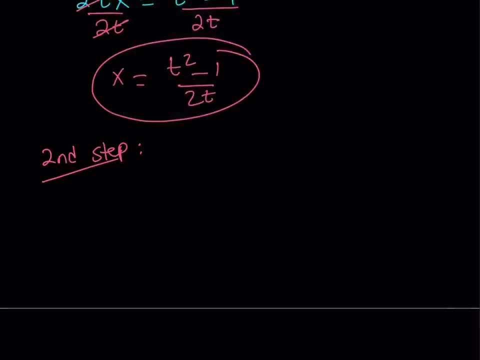 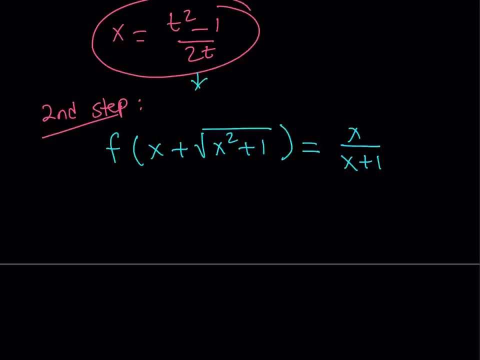 our original expression looked like right. Our original expression looked like the following: f of x plus the square root of x squared plus 1, and that equals x over x plus 1.. Okay now, what am I going to do? I'm going to use this expression here. I'm going to replace x with t squared minus. 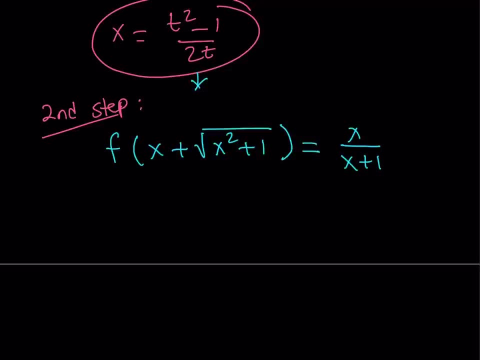 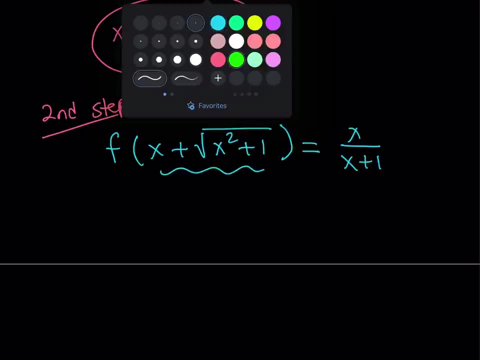 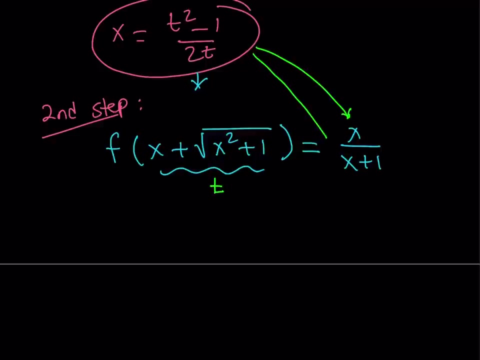 1 over 2 t on both sides. but when I do it on the left hand side, inside the parentheses, I already know that it's going to give me a t here, because that was my original substitution right. So I do know that this is going to be a t automatically. so what I need to do is replace the x with what it. 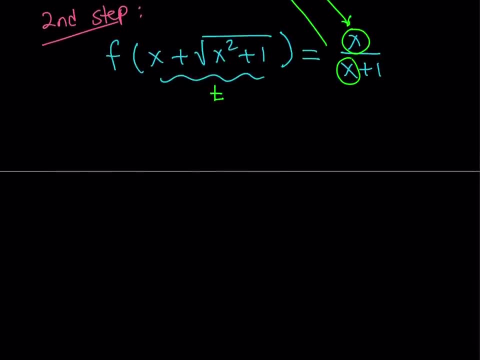 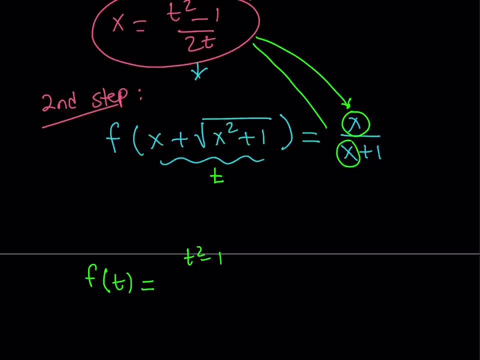 is on the right hand side. Let's go ahead and do that. So this gives us f of t is equal to x, which is going to be replaced by t squared minus 1 over 2 t over t squared minus 1 over 2 t plus 1.. 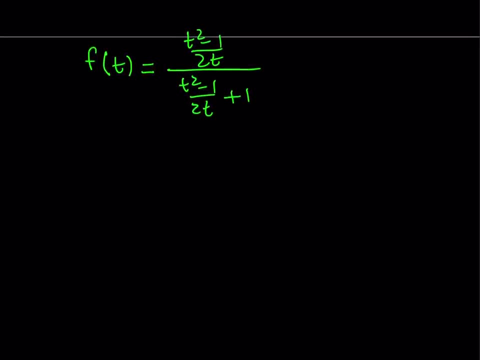 Okay, so this is my f of t. Let's go ahead and simplify this, and when you're trying to simplify these kinds of things, it's pretty much the same thing, but I would like to, instead of making a common denominator, I would like to multiply the top and the bottom by 2t, because I believe it's. 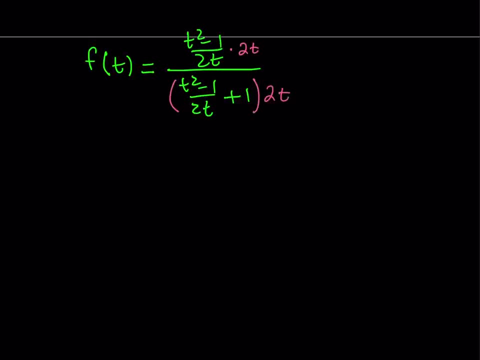 going to take us to the result faster and from here we're going to be getting: f of t is equal to 2t is going to cancel out t squared minus 1 in the numerator and the bottom, when you distribute to 2t, 2t is going to cancel out. it's going to leave us with t squared minus 1. 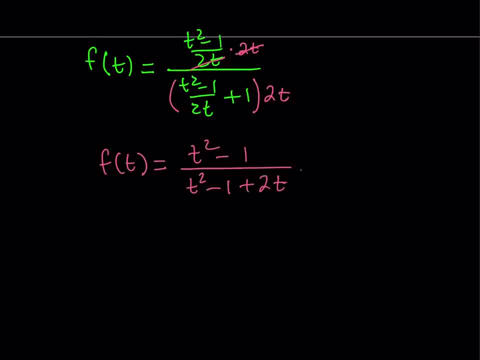 and 1 times 2t is 2t. Obviously, I can write it as t squared minus 1 over t squared plus 2t minus 1.. Of course, I do want to find f of x, so let's go ahead and replace t with x on both sides, which. 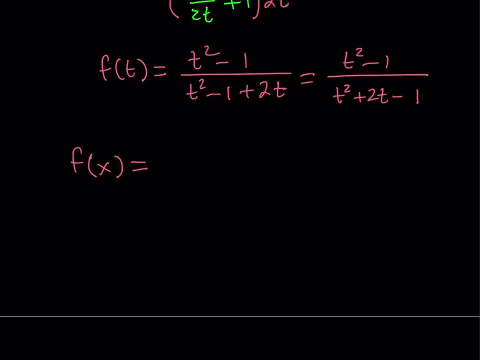 is a very easy step to do, because you can use pretty much any variable on both sides of the equation as long as you use the same variable. So now replace t with x, and this is going to give us f of x. So let's go ahead and do that. So let's go ahead and do that. So let's go ahead. 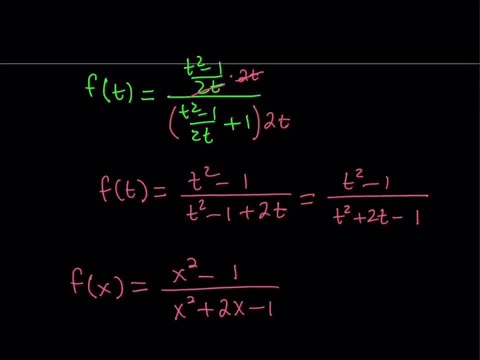